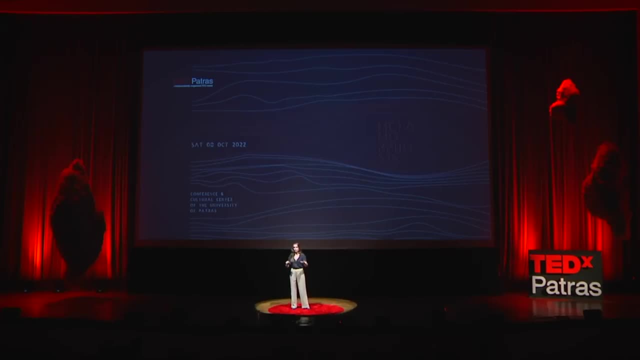 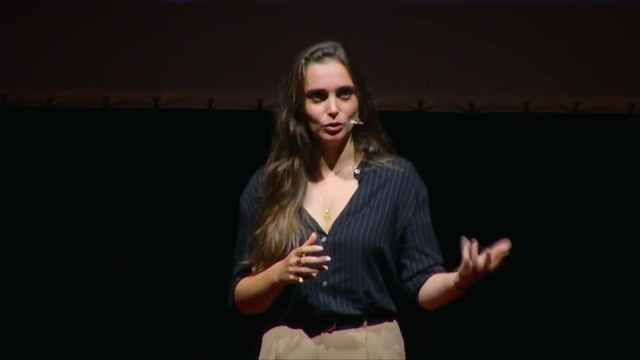 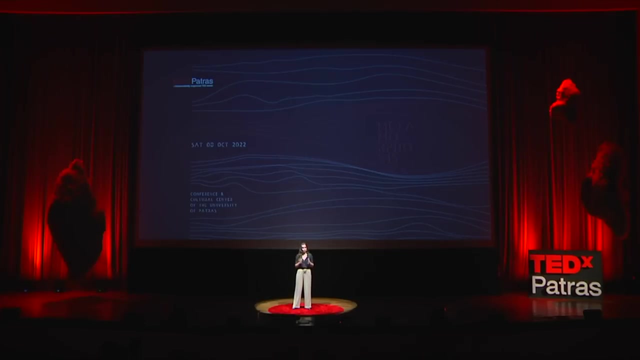 has an input that produces an output that can be sent to other nodes. This all functions like a biological neuron. Neural networks are a reflection of how our human minds interact with information in the world around us. Data sets. Data sets are a collection of information points on human habits and activities. Everything. 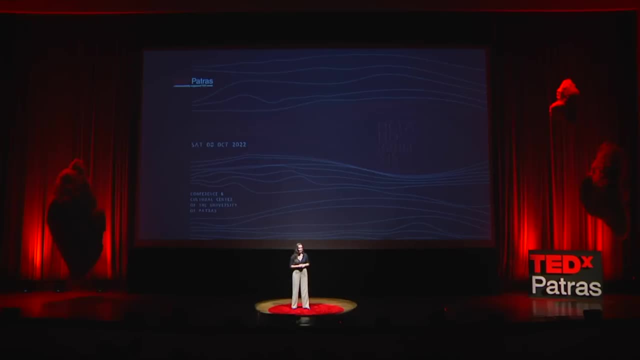 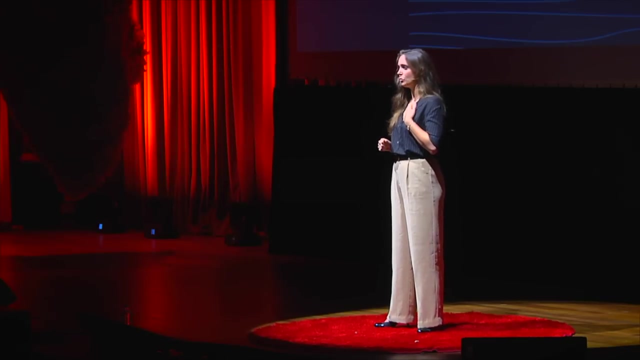 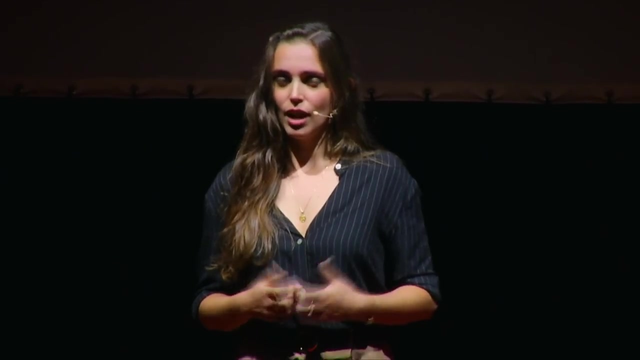 from how often in a year you actually floss, to how your eyes move across the screen, to how fast your heart beats when you're looking at someone you love. Data sets are a collection and a reflection of how our human behavior forms patterns in the world around us. 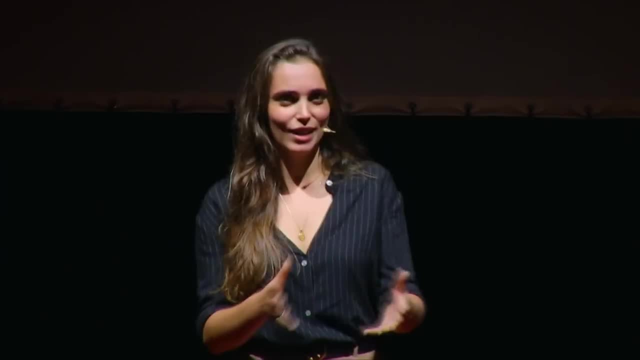 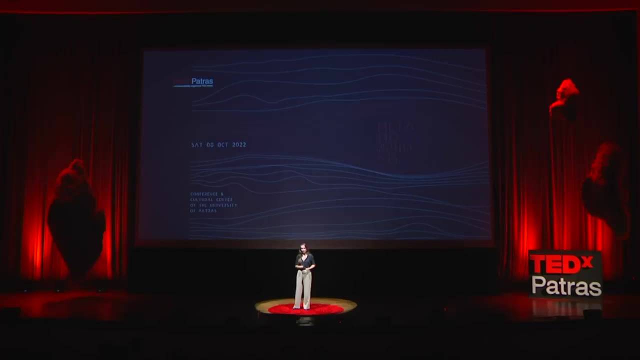 So you see, our technology is not some grand, mysterious thing outside of our comprehension and control. Our technology, at its most basic level, is a reflection of our humanity. Which leads me to my next question: What does it mean to be human? 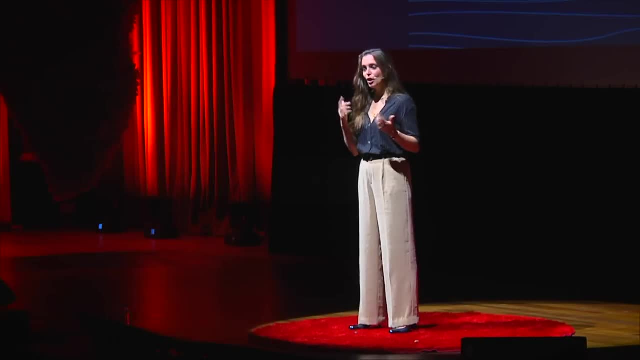 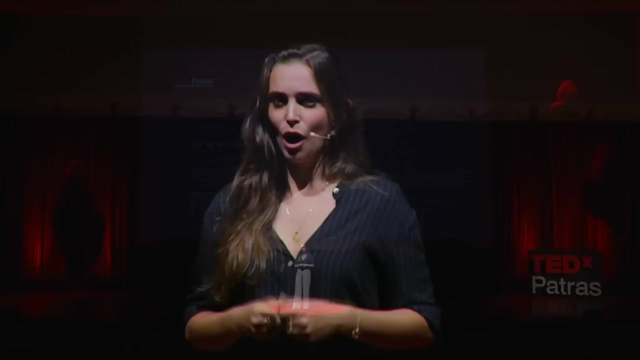 So far, we've covered our mind, our body, our behaviors, But is this all there really is to being human? What about our emotions, those messy feelings? our dreams and aspirations, our ability to believe in something and to have the strength to stand for it? 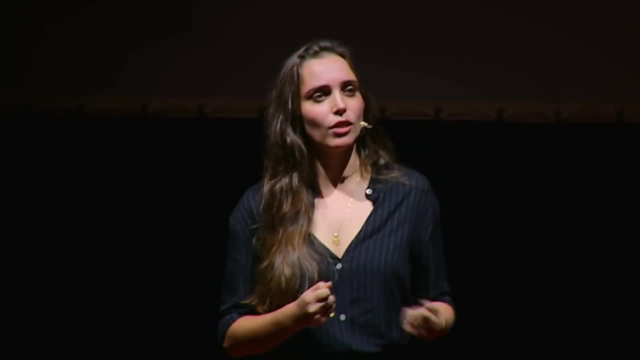 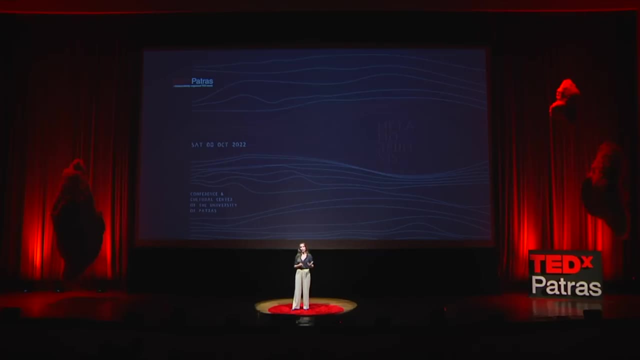 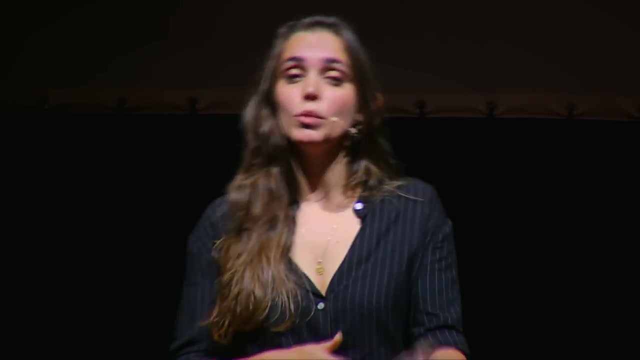 What about love and our need to cherish the connections with those around us? To be human means to have values and to build our life on these values. We, as humans, are innately moral creatures, And if our technology is supposed to be a reflection of our humanity, 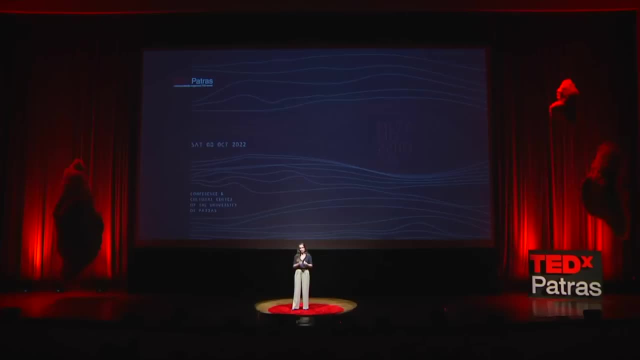 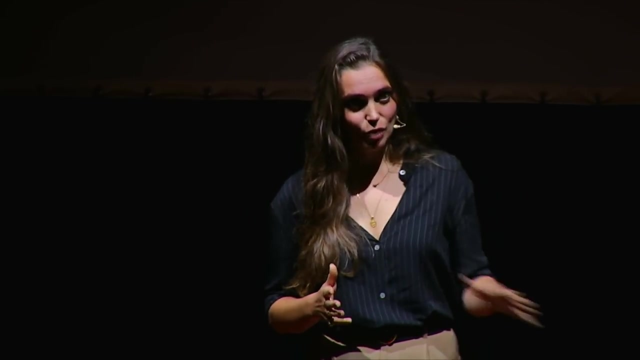 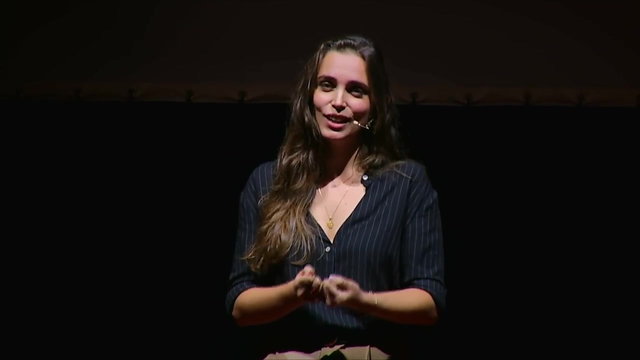 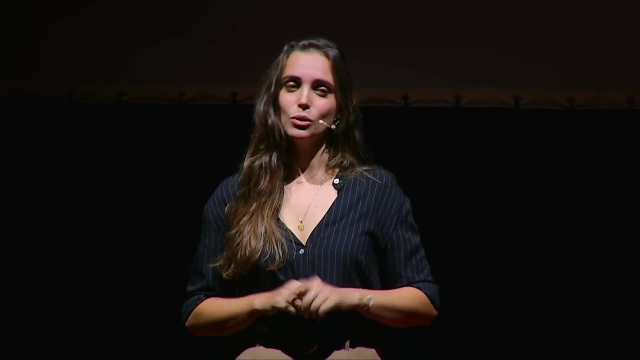 then, why does our technology today miss this crucial element of our humanity? Well, it's all because somewhere along the way, we forgot about one of the most powerful tools we have as humans in creating and building a life and technology of values. This tool is ethics. 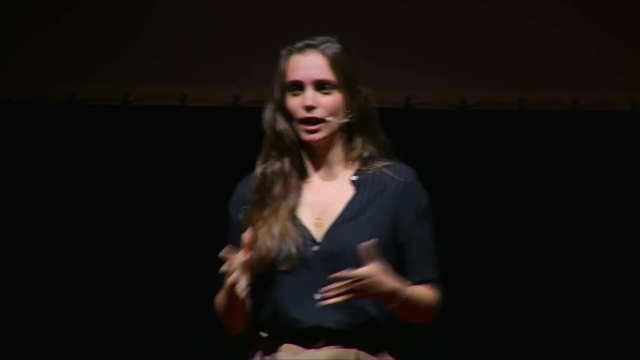 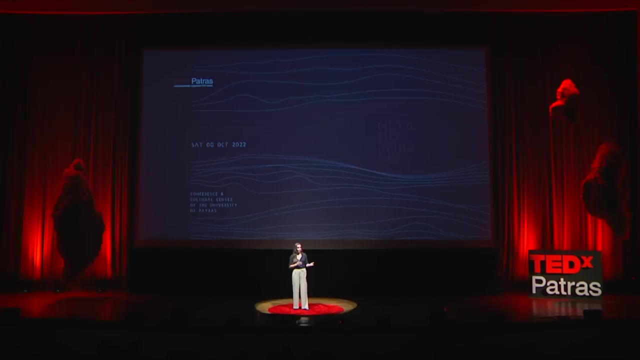 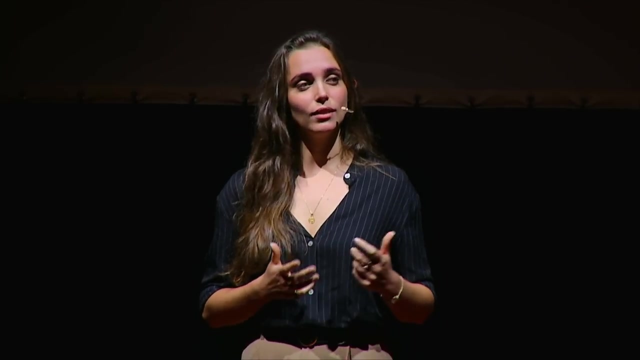 Allow me to explain by first looking at how we use ethics in our daily lives as humans. I want you all to take a moment and ask yourselves: what is a good life? What would it mean to live this life? What would that even look like? 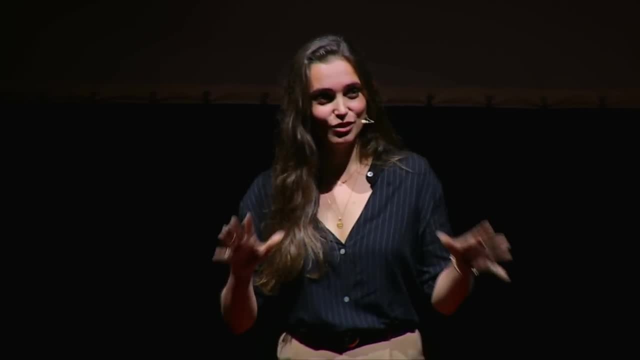 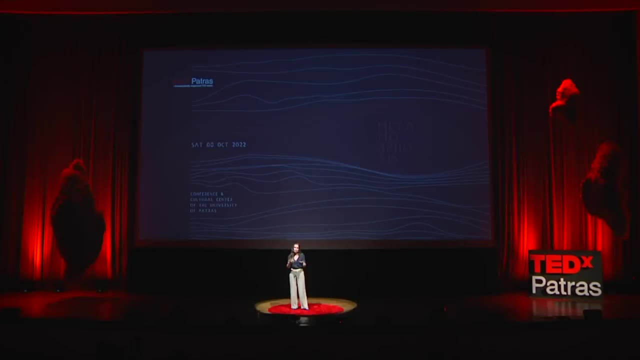 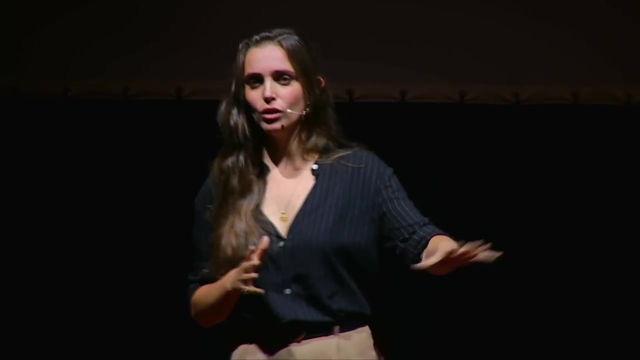 Now I can guarantee you that there are hundreds of different good lives being pictured in this room at this very moment, But the beautiful thing is that, even though we may all have a different conception of what it means to live that good life, all of our good lives share a common thread. 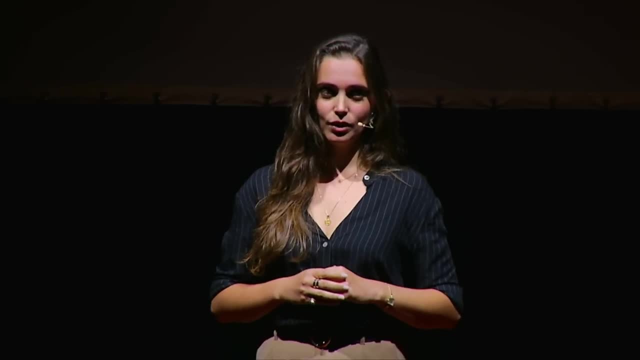 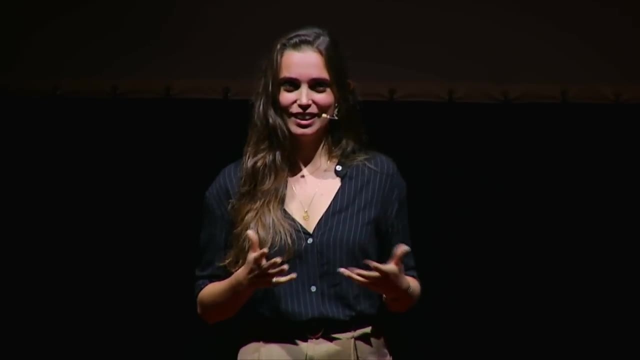 Details aside, what you're picturing right now is a fulfilling life of purpose. Although there may be elements of the dolce vita, a good life at the end of the day is one that you can sit on your deathbed with a sense of peace. 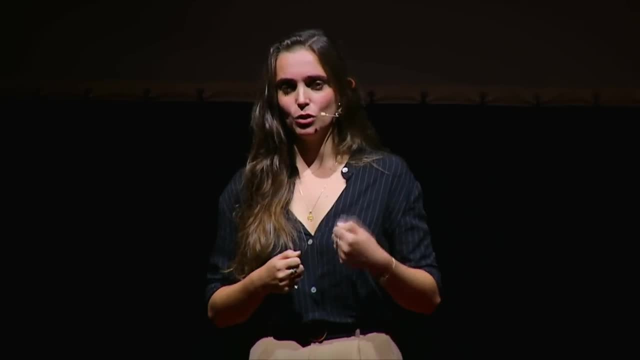 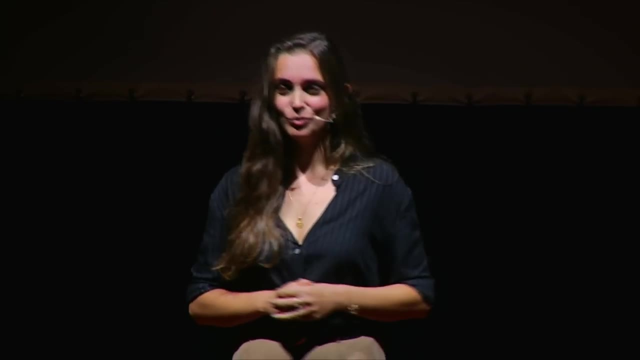 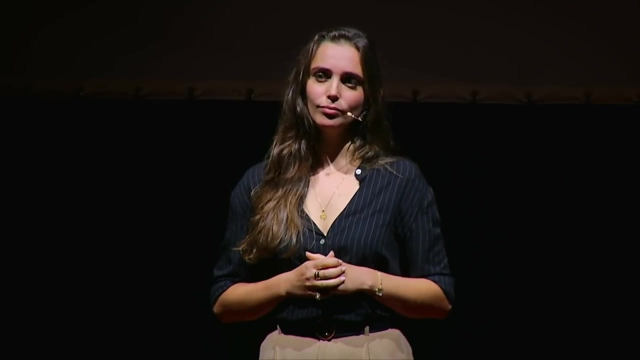 knowing that you've found fulfillment, that you fulfilled your purpose. Where do we find this purpose, though, In this life? our purpose is found in the values that define us, Whether these values be love of family, freedom to speak and be heard. 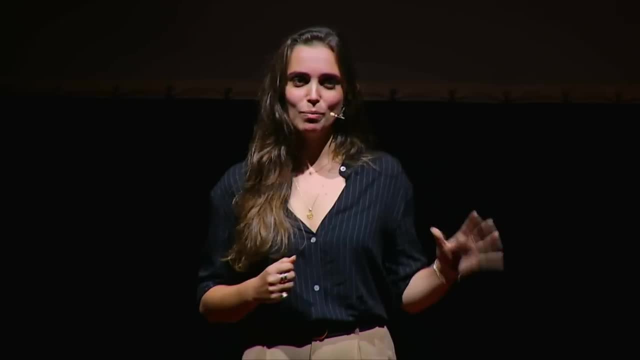 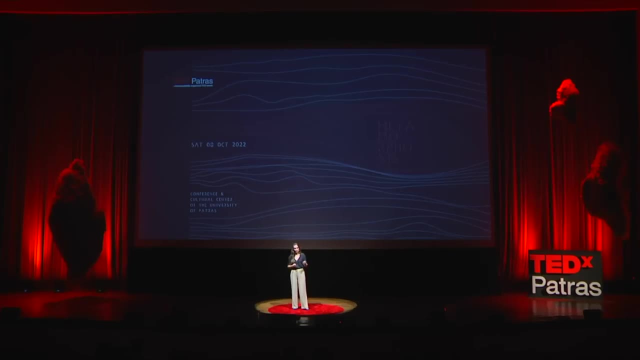 resilience in the face of seemingly unmovable mountains. our values come in so many shapes and sizes, But at the end of the day, what makes a value is the conviction to say: here I stand and you won't move me. Now, how do we live this life? 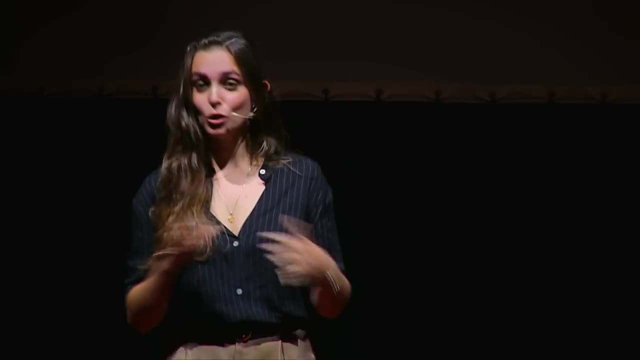 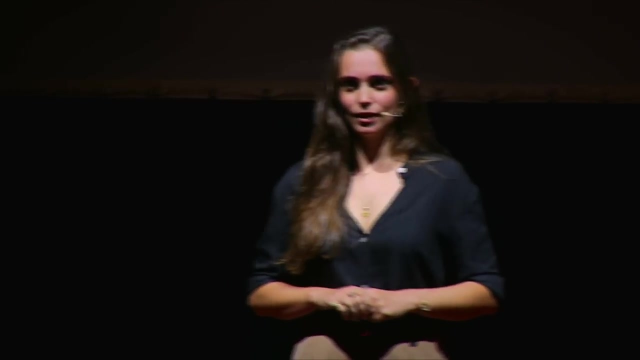 In theory sounds beautiful, but I'm sure we can all agree it's not as straightforward as we would hope. It's easy to get lost in the day-to-day. It's easy to forget that we're here to fulfill a purpose. It's easy to forget. 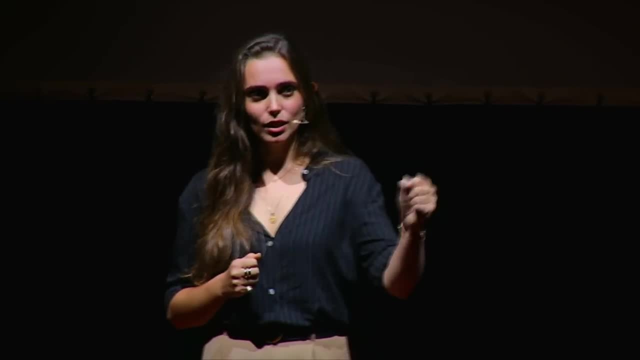 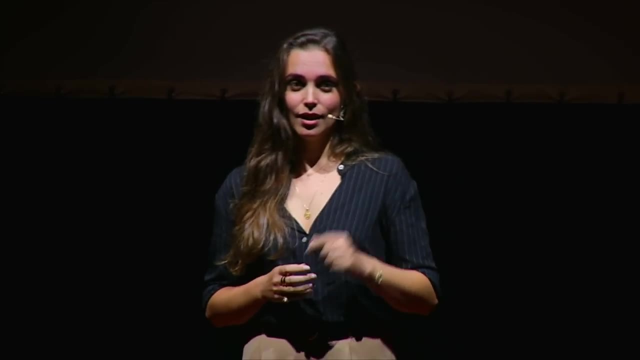 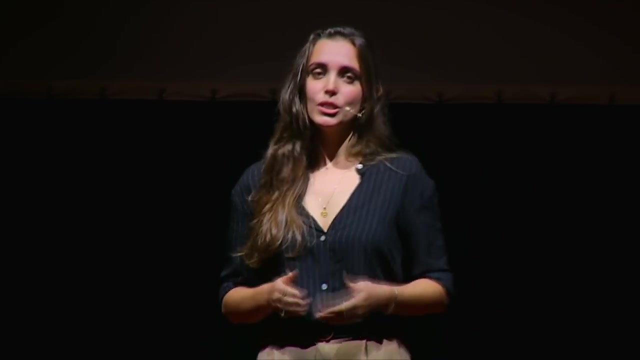 that the good life is always within reach. It's just a few good decisions away. This is exactly where ethics comes into the equation. You see, at its root, ethics is a reflexive tool that we are constantly using in our daily lives. 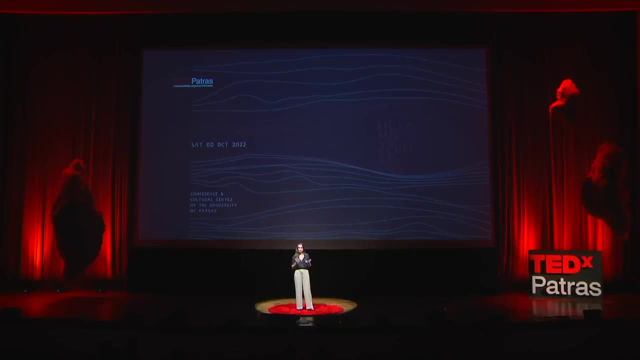 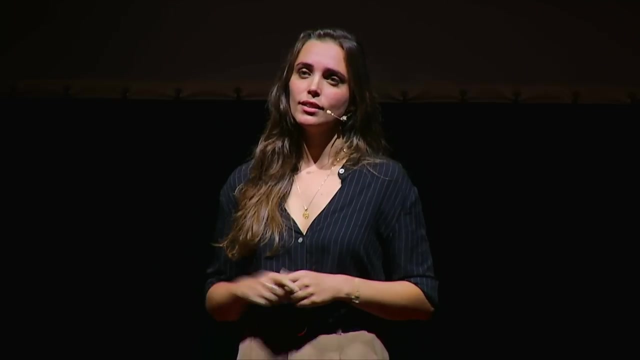 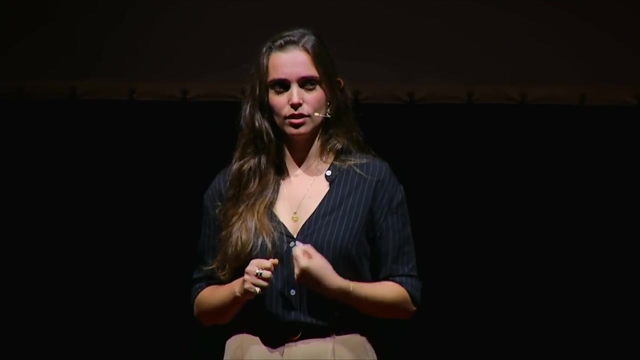 Sometimes it's consciously As you sit and decide whether or not to bail your friend out of a financial crisis. if you'll join that protest against that law that you disagree with, if you'll join that organization for that cause that sits at your core. 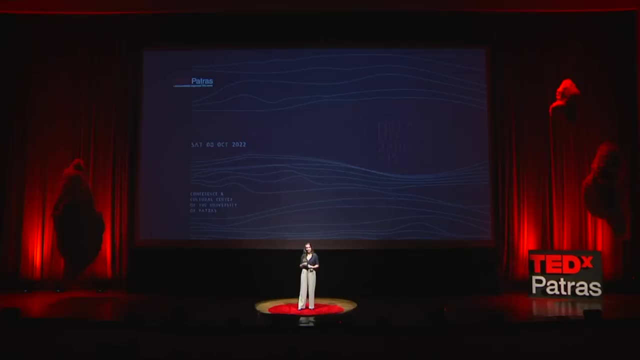 And sometimes ethics is unconscious. It's that gut instinct that causes you to act in a split second, to throw yourself in front of a car to save that child, to offer the homeless man on the corner your jacket on a cold night, What you're doing at either end of these extremes. 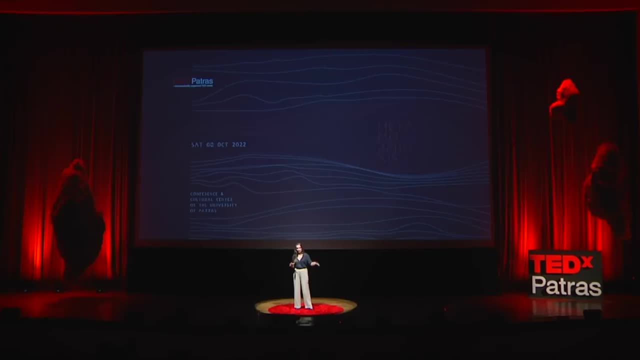 and everything in between is using ethics as a tool in the pursuit of your good life. If a good life is a life in which your actions reflect your values, then the opposite of this life is a life in which you have no values, or even worse. 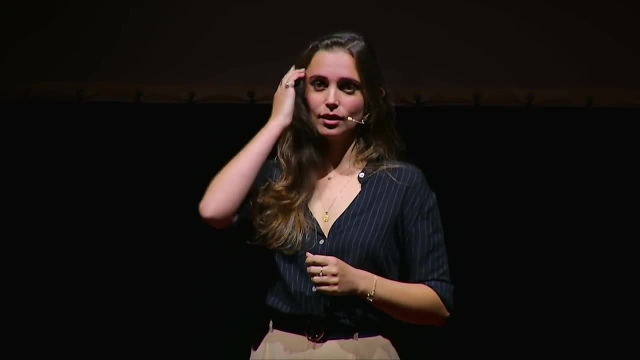 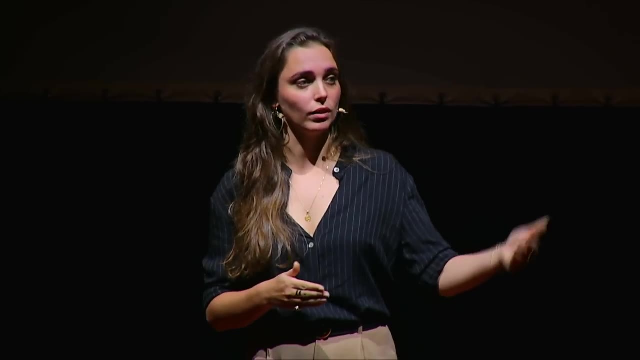 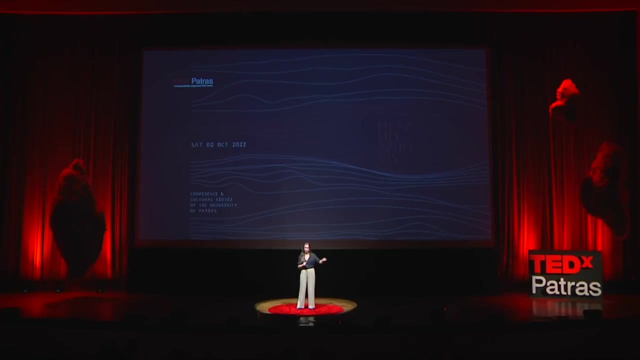 actively go against these values. You see, ethics is the tool we use to reflect and determine if our actions are in alignment with our values. Think of it this way: Your purpose is like an end destination on a map. Your values are the directions. 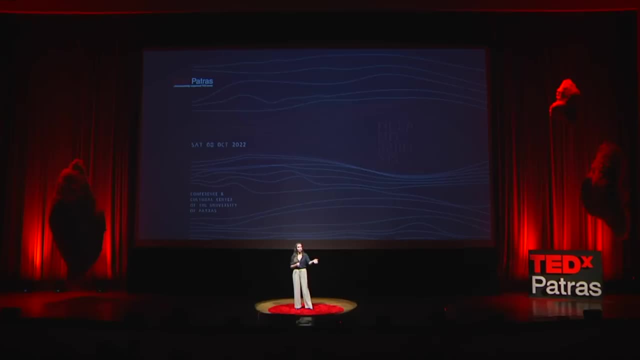 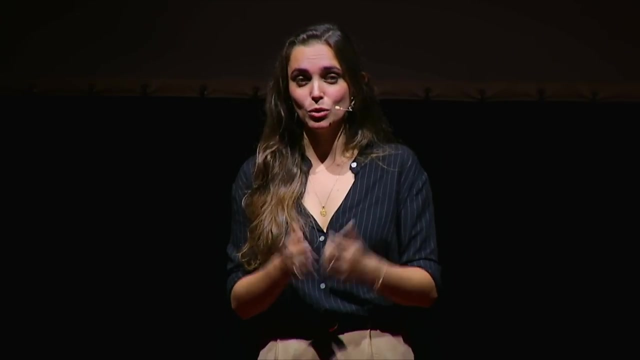 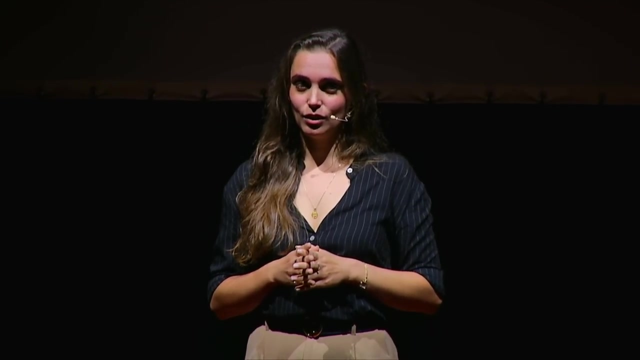 you need to follow to reach that destination. And ethics, That's the compass. That's the compass that allows you, enables you to follow those directions to reach your final destination. Remember how I said: a good life is always within reach. just takes a few good decisions. 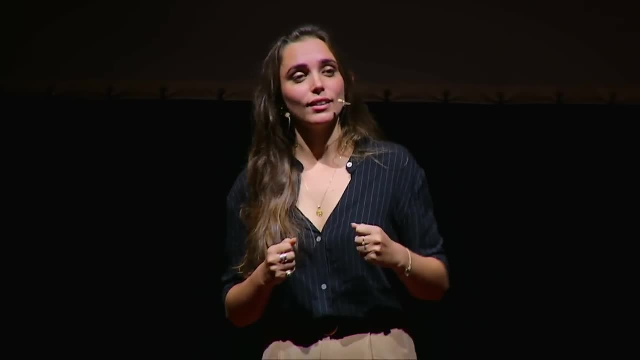 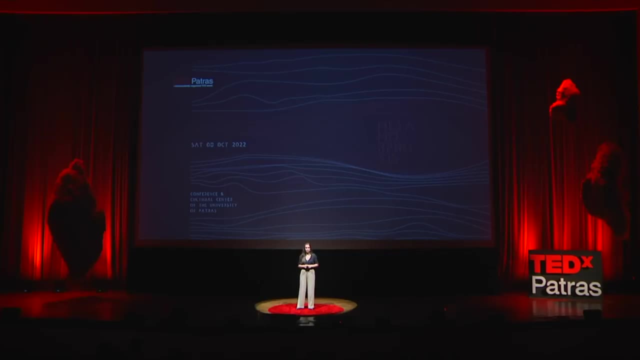 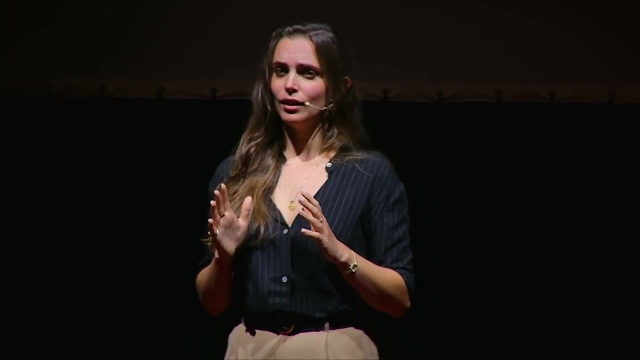 What I mean by this is if we use ethics to guide our decisions in a way that aligns our actions with our values, that's fulfillment, That's purpose. That's practicing ethics. Now, what in the world does this have to do with technology? 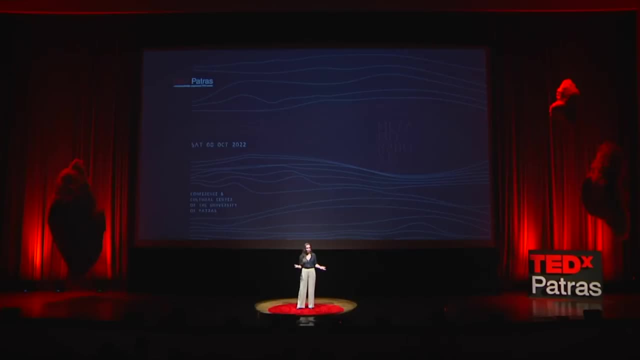 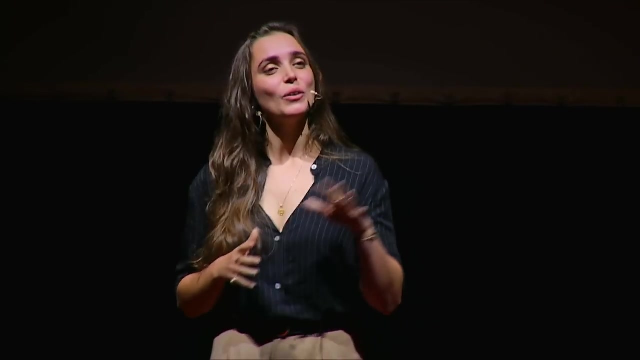 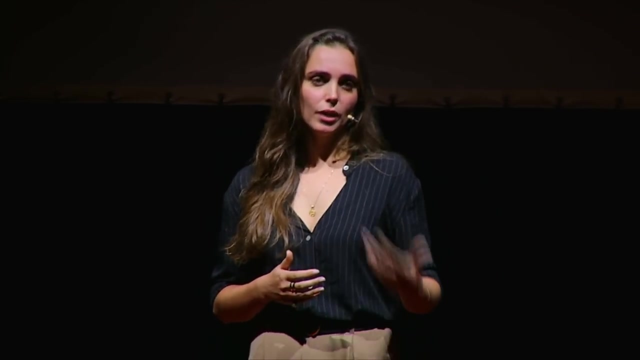 Probably sitting here going. I like values, I like a good life, But weren't we supposed to talk about tech? Well, you see, our technology is a reflection of our humanity. And now that we understand how to use ethics on the human level, 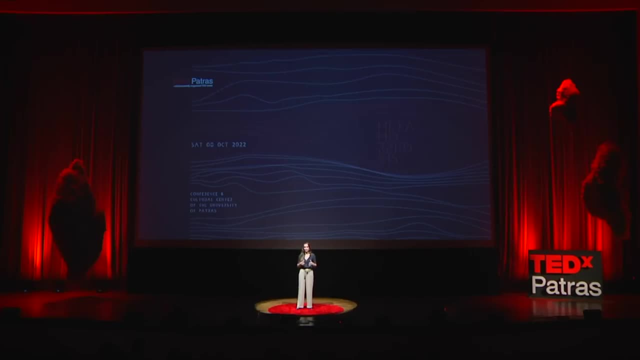 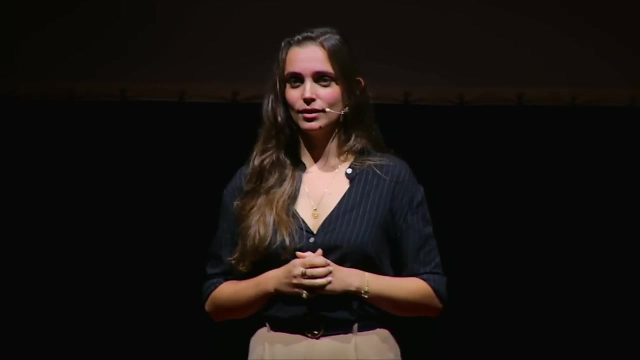 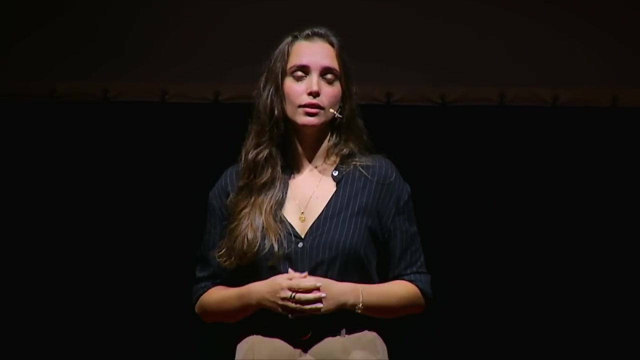 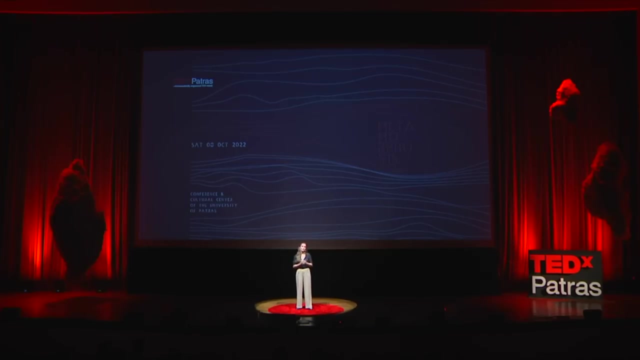 we can start to look at how to use ethics on the technological level. And I'm going to start with the same question: What is good technology? What does it mean for tech to be good? What would this even look like? Is it a social media network? 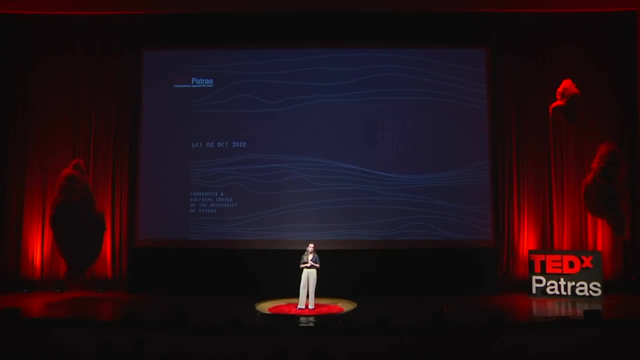 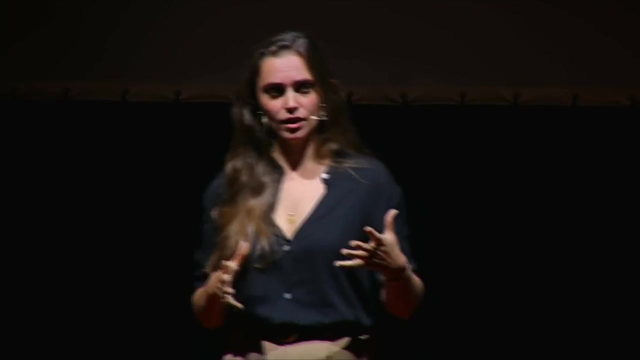 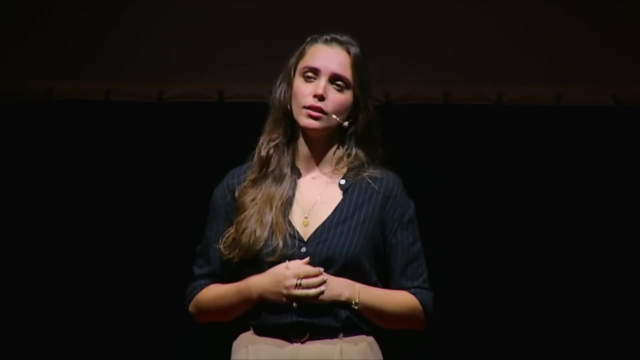 designed to capitalize on our insecurities and thrive off of content full of hate and anger? Is it a health app that tracks every single one of our movements, whether we know it or not, only to take that information and sell it to insurance companies? 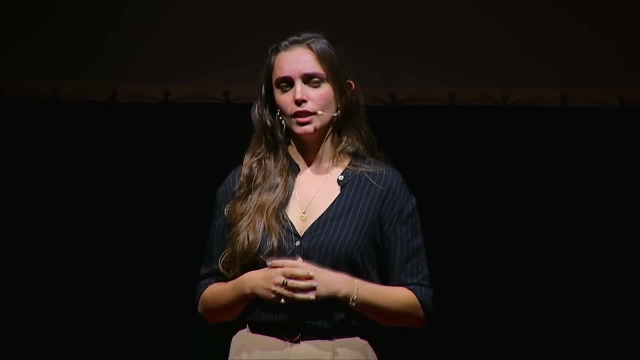 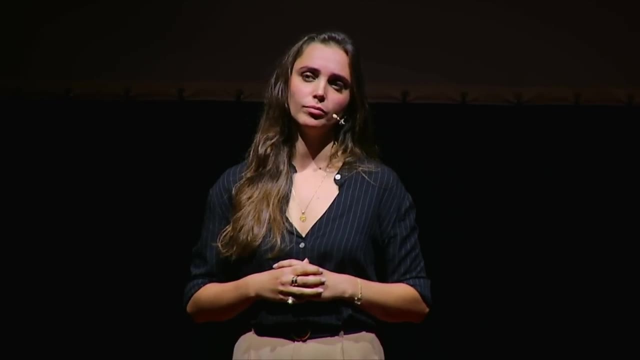 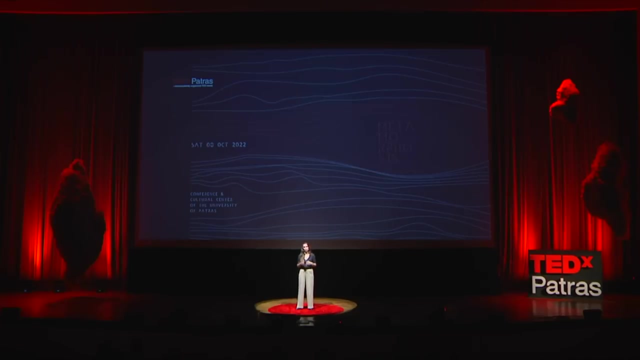 Is it a credit scoring algorithm that takes the zip code you were born in to determine how likely you'll be to default on a bank loan? Is it a HR hiring software that, despite your best efforts, can tell your gender based off of the adjectives? 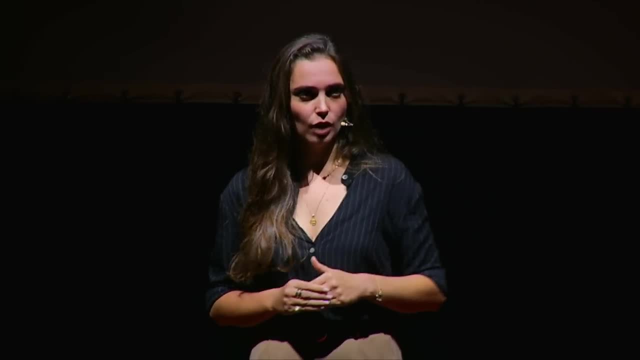 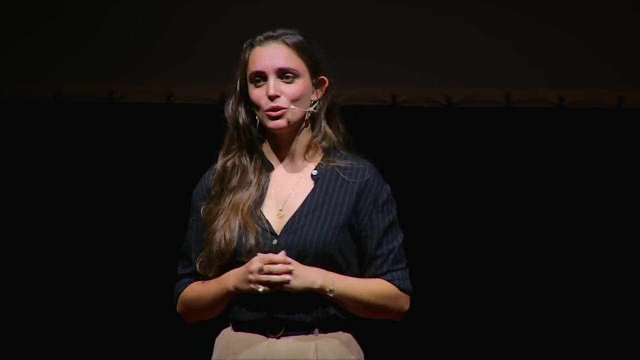 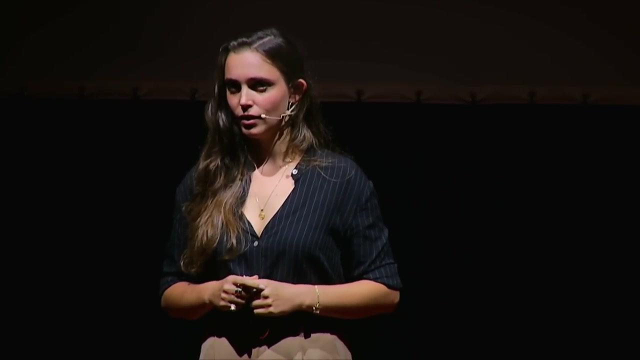 you use to describe yourself and whether or not you'll be a good fit for that role. Is it a recommendation system designed to pursue profit at the very cost of dignity of the individual? Is this good tech? Because this is the technology that we have today? 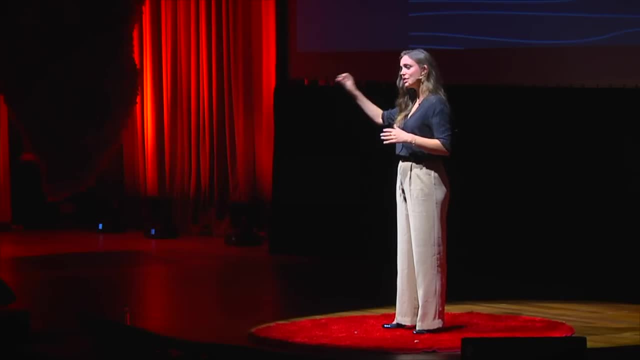 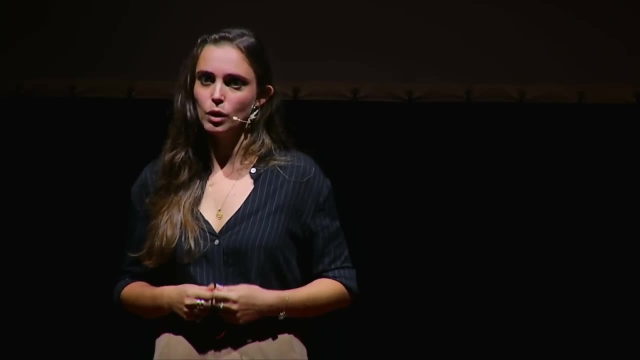 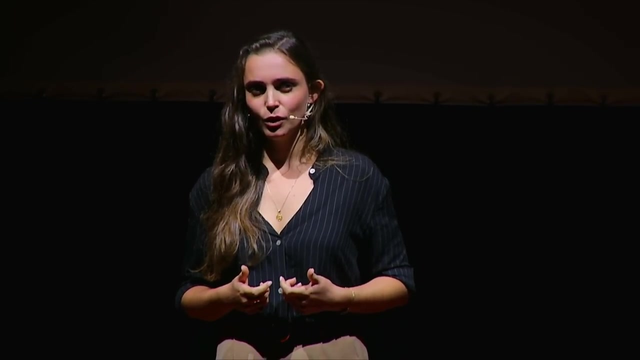 This is not some tech that we're building in the future. This is technology that we have built and are using. Is this good tech? Is this really what we wanted? No, Of course not. We as humans are so much more. 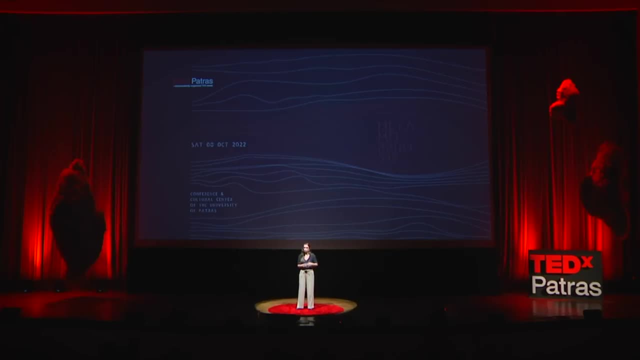 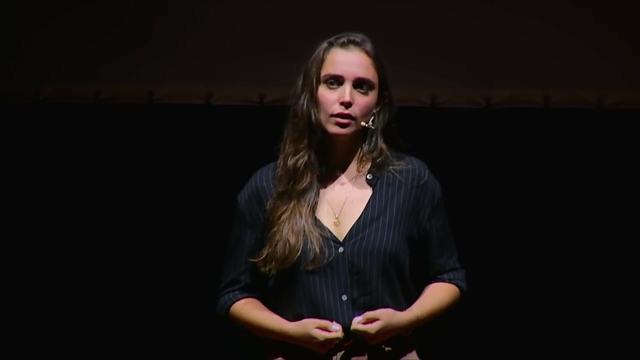 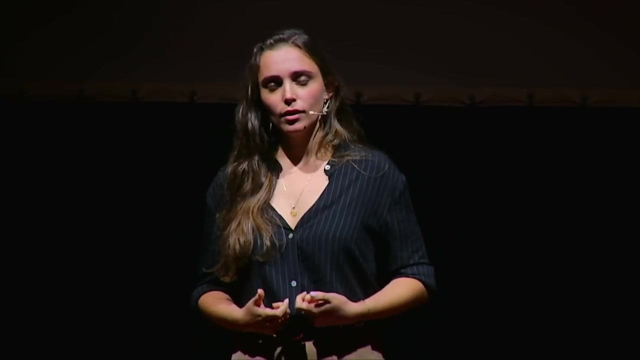 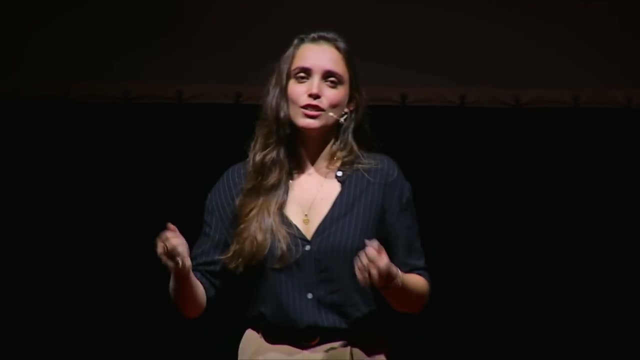 than micropayments and privacy invasions and social scoring and bottom lines, and filter bubbles and structural bias. We are more And we deserve technology that is more. You see, good tech is not technology that takes advantage of our human nature. It's technology that helps us embrace. 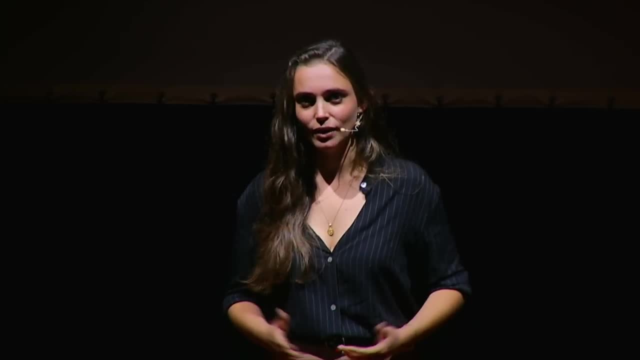 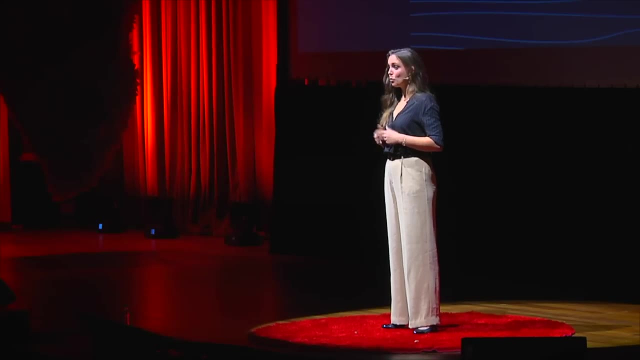 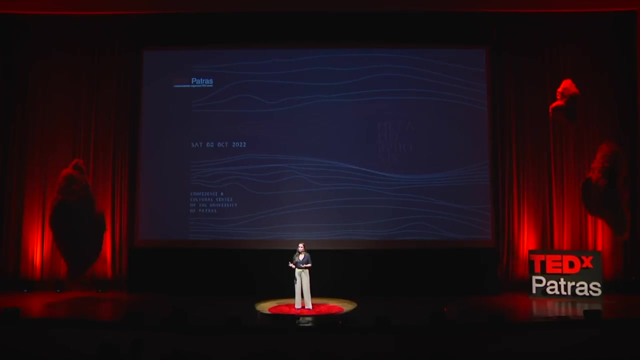 the nature of being human, And we as humans are innately moral creatures. We have values And we find fulfillment in life. We find our purpose in these values, Which means our technology needs to be able to support and enable and empower us. 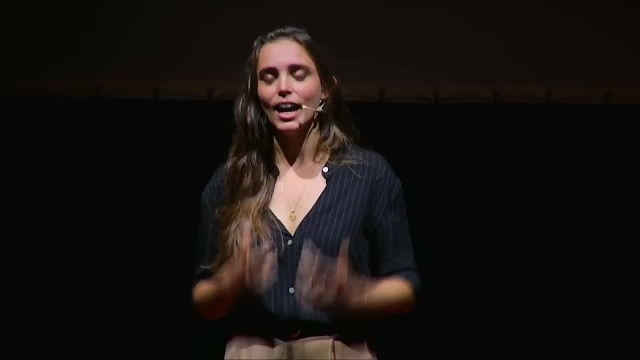 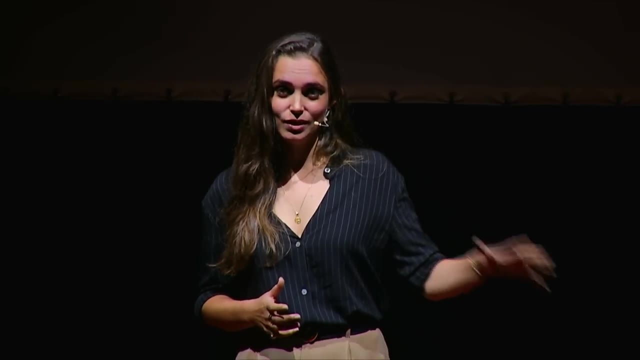 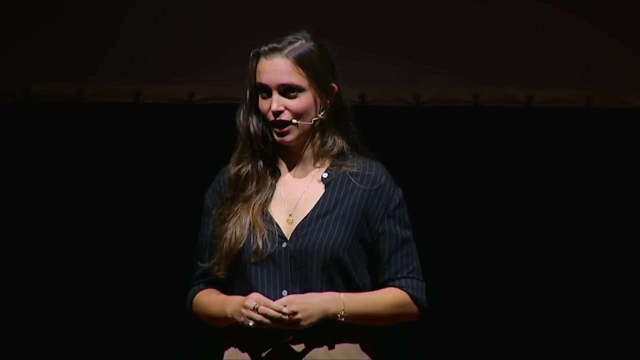 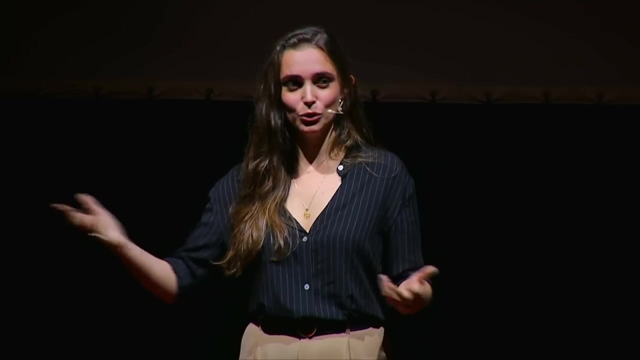 to live in alignment with these values. That is good tech, And it's only a few good decisions away. But we've forgotten about in our development of our technology today what's kept us from the pursuit of good tech. We forgot about our most powerful tool. 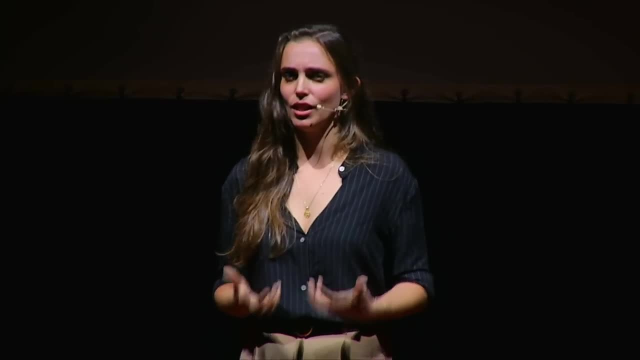 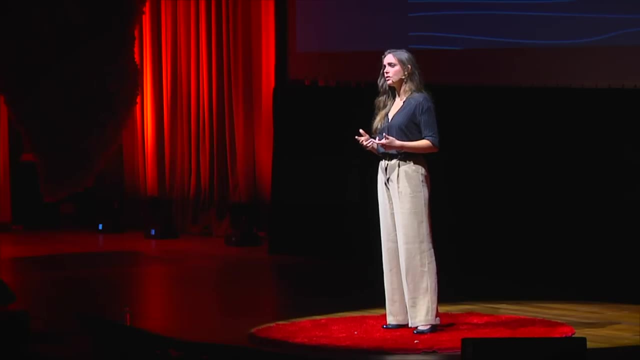 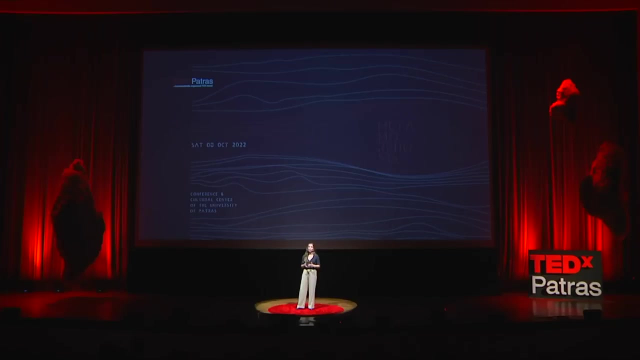 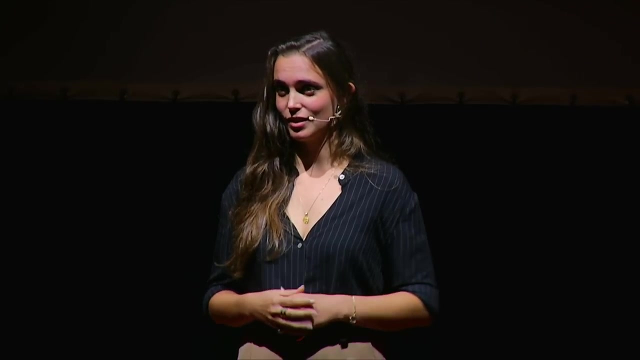 We forgot to pause and critically ask ourselves if what we're building is helping or hindering us. We forgot to reflect on our habits and how we engage and use technology in our daily lives. We forgot to align the purpose of our systems with the values as we hold as humans. 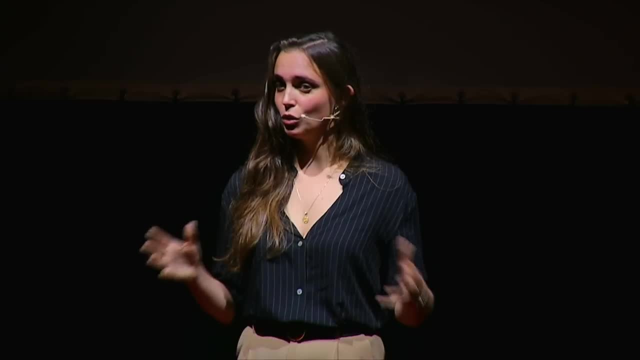 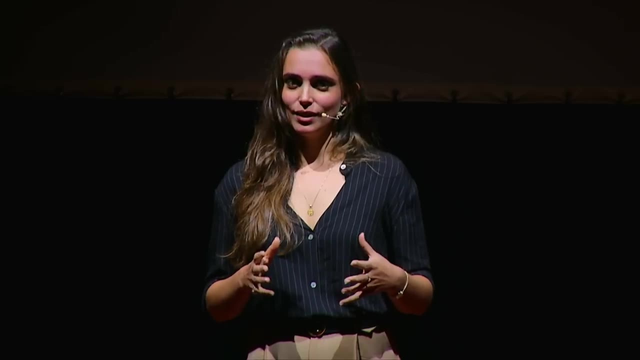 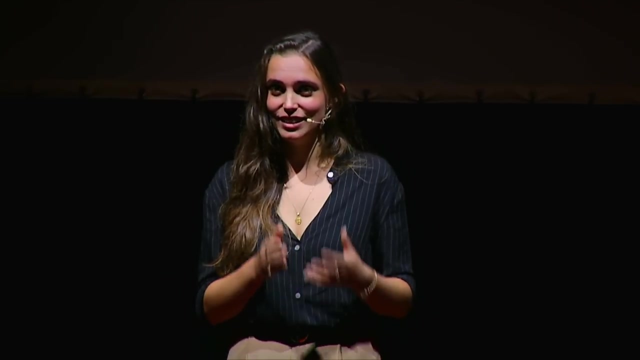 Somehow, somewhere along the way, we forgot all about ethics. Now I want you all to take a moment and ask yourself what would this world look like if we actually used ethics in the design and development of our technology? What would it mean to align our tech to our values? 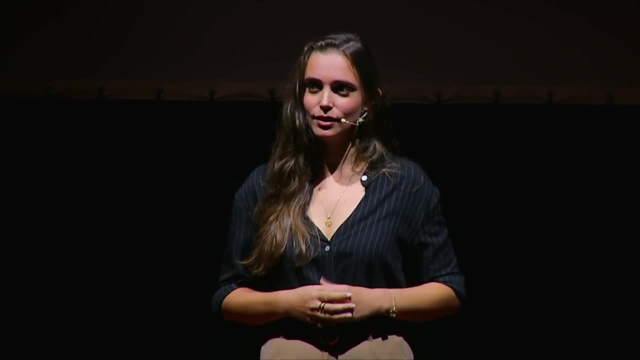 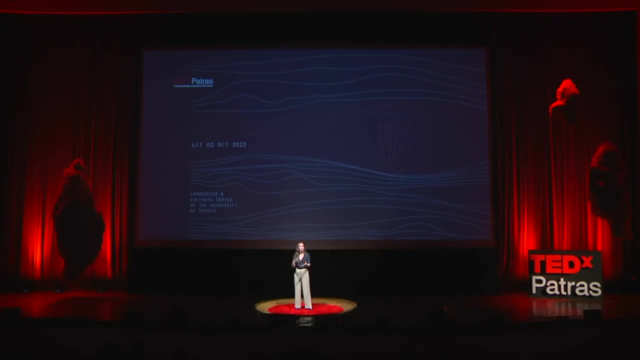 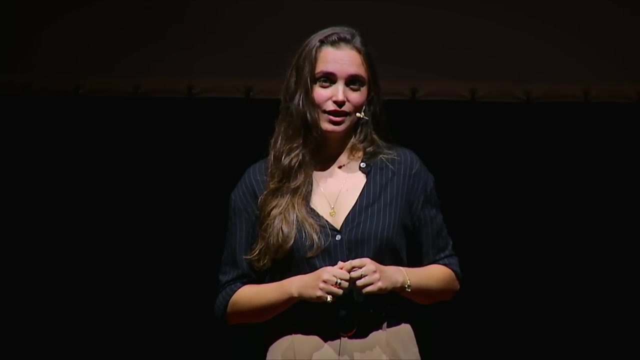 What would this world look like? It would look like a world full of genuine human connection, where our technology brought us closer together instead of driving us further apart. It would look like a world in which we all had the freedom to chase our full potential. 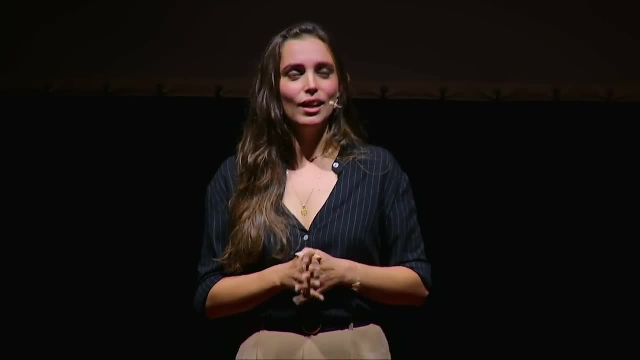 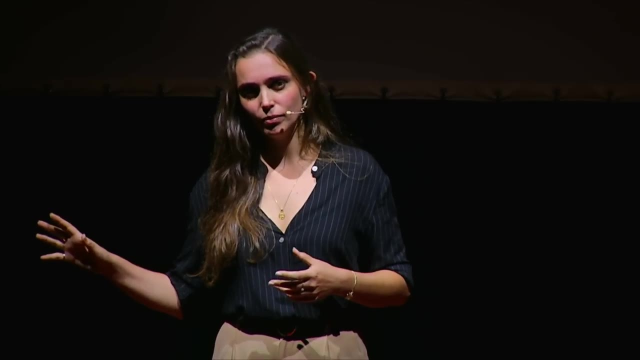 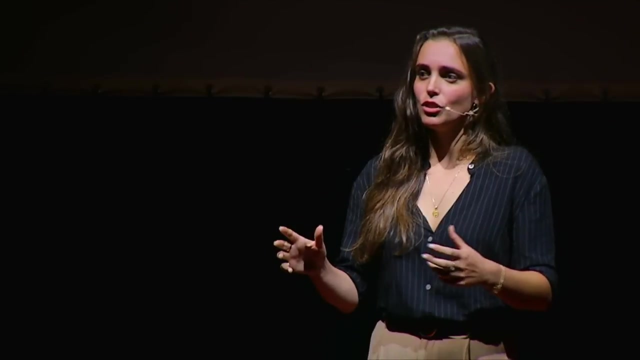 no matter the circumstances we were born into, In which technology opened up new avenues for success instead of leaving our fate up to an algorithm. It would look like a world in which we could rely on each other, In which technology fostered open communication instead of overbearing surveillance.